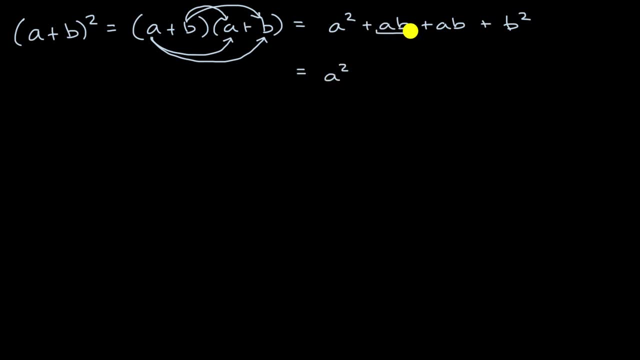 But this is going to simplify to a squared plus. we have an ab and another ab, so you add those together, you get two ab plus b squared. Now why did I go through this review? Well, now we can use this idea. 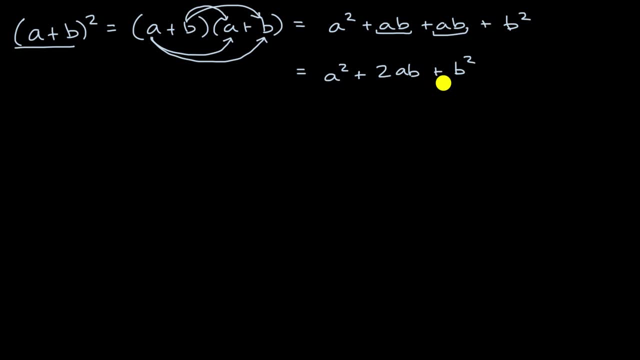 that a plus b squared is equal to a squared plus two, ab plus b squared, to tackle things that at least look a little bit more involved. So if I were to ask you, what is five x to the sixth plus four squared? pause this video and try to figure it out. 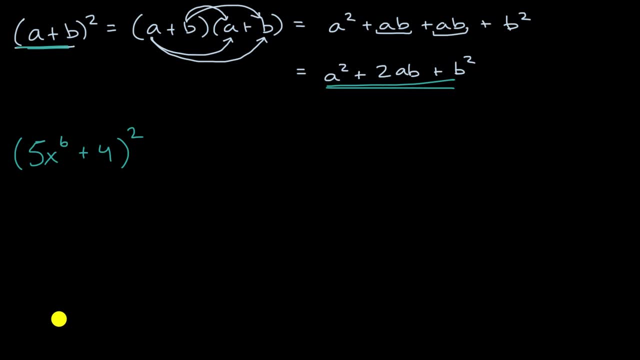 and try to keep this and this in mind. well, there's several ways you could approach this. You could just expand this out the way we just did, or you could recognize this pattern that we just established: that if I have a plus b and a squared, 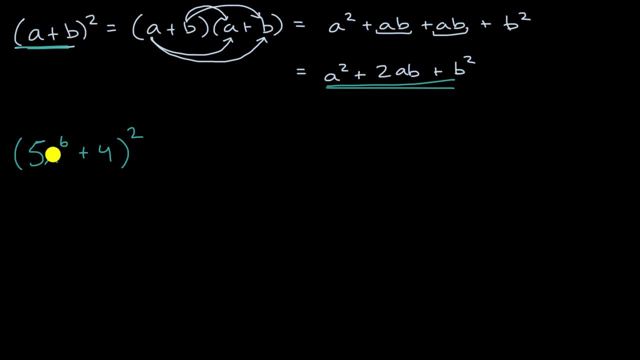 it's going to be this, And so what you might notice is the role of a is being played by five x to the sixth right over there, And the role of b is being played by four right over there. So we could say, hey, this is going to be equal to. 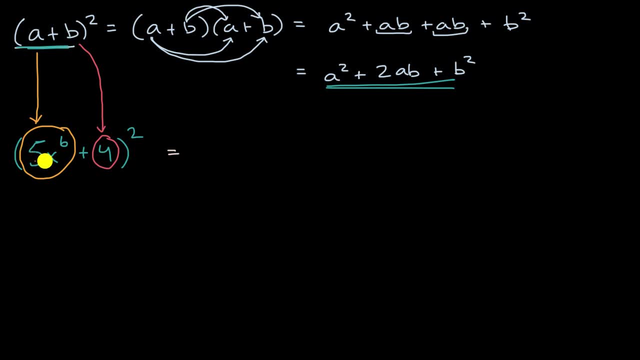 a squared. we have our a squared there. So what is a squared? Well, five x to the sixth squared is going to be 25 x to the 12th power, And then it's going to be plus two times a times b. 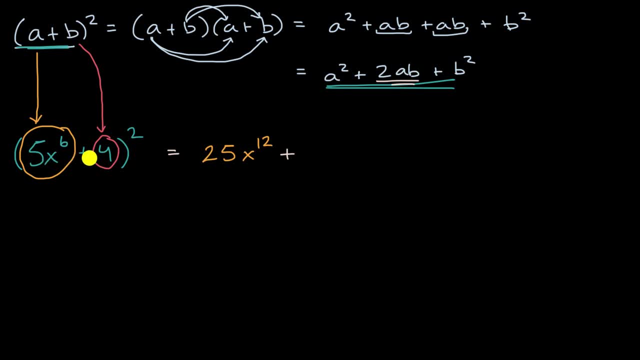 So plus two times five, x to the sixth times four. Actually, let me just write it out, just so we don't confuse ourselves: Two times five, x to the- I'll color code it- two. Two times five, x to the sixth times four. 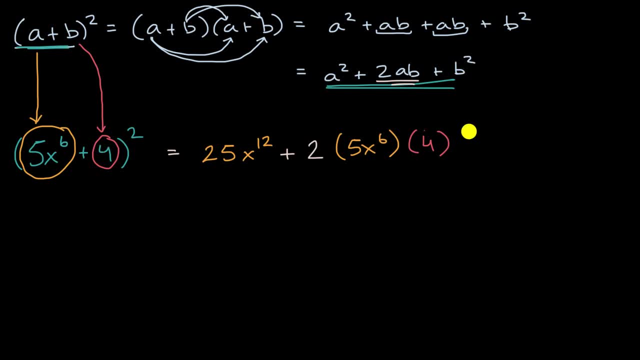 times four plus b squared, So plus four squared, so that's going to be plus 16.. And then we can simplify this. So this is going to be equal to 25 x to the 12th. Two times five times four is 40.. 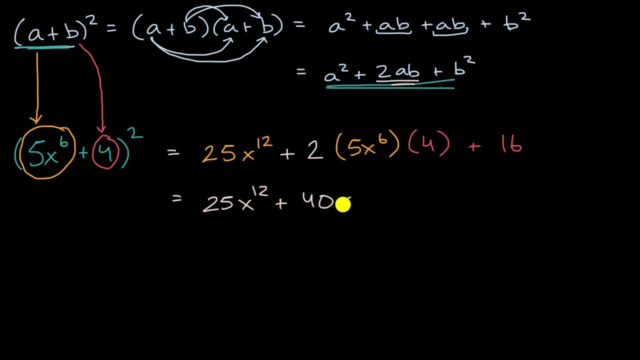 Two times five is 10.. 10 times four is 40. So plus 40 x to the sixth, plus 16.. Let's do another example, And I'll do this one even a little bit faster, just because we're getting, I think, pretty good at this.